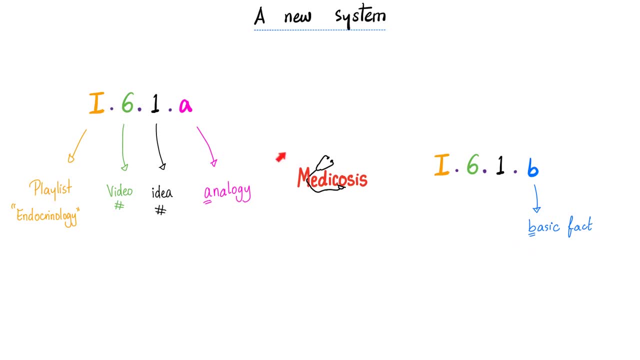 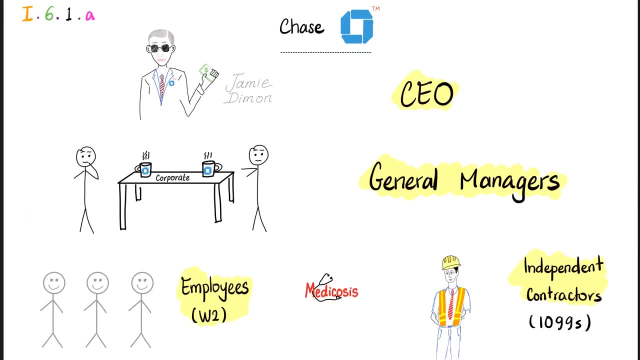 If you understand the analogy, you will get the basic fact And then, at the end of each video, try to think: how many facts did we include? and try to recall, because it trains your memory. Analogy number one: Any company has what Jordan Peterson might. 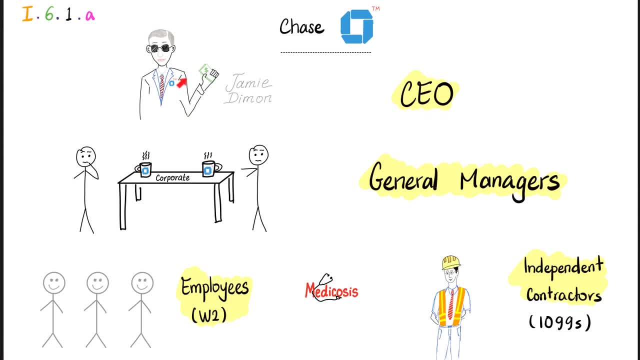 say, a dominance hierarchy starting by the chief executive officer, Then you have general managers and then you have two groups of people: The employees- they are hired by the company, They are part of the staff, They have to obey every commandment. and the independent contractors. 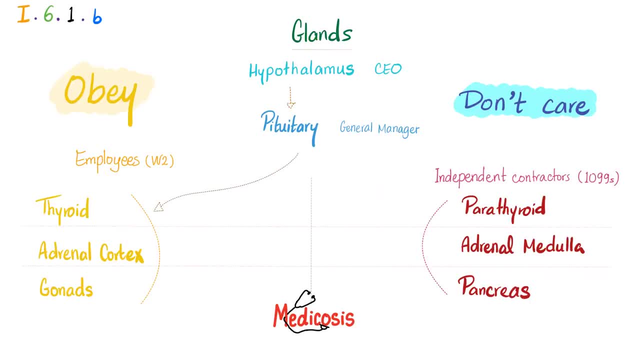 Your endocrine system is the same: The CEO is the hypothalamus, The pituitary is your general manager, And then you have the employees thyroid, adrenal cortex and gonads. These are the people who obey the pituitary, especially the anterior pituitary, And then we have three people who 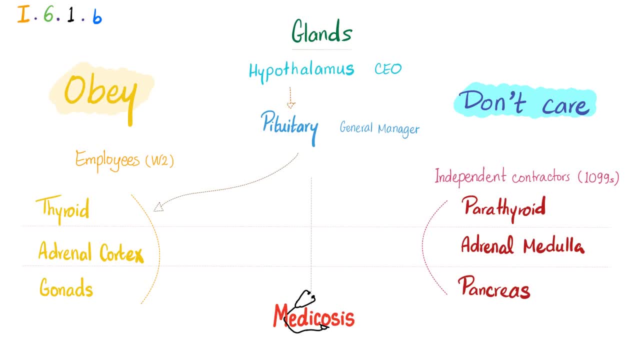 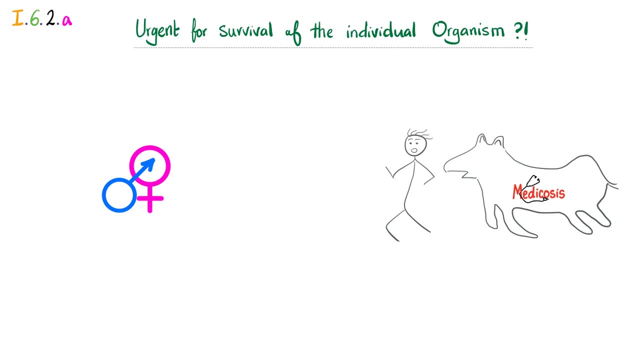 could not care less about the pituitary, And these are the parathyroid, adrenal medulla and pancreas. Analogy number two: Okay, which one of these two activities is most important or most urgent for survival of the individual organism? You running from a tiger or you participating in? 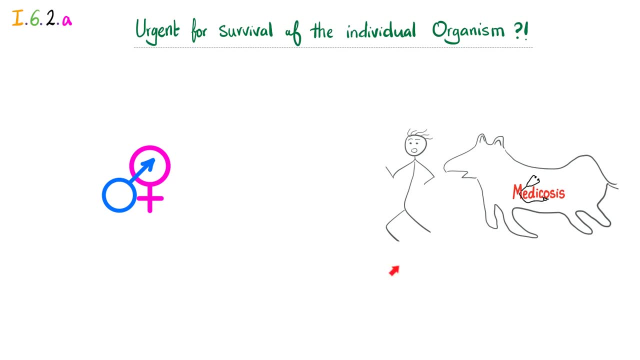 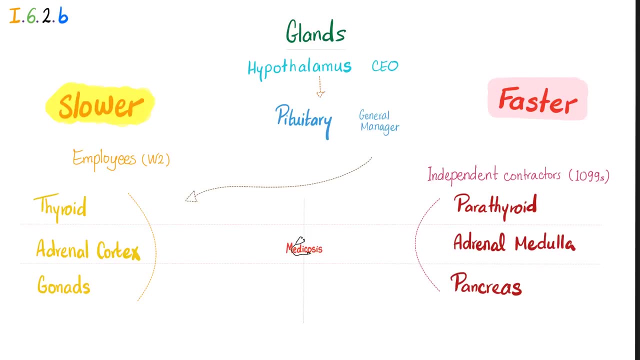 coitus, I gotta keep it G-rated for the algorithm, Of course. running from a tiger- Oh, this is gonna be. oh, yeah, of course, this is more important, This is more urgent When you're running from a. tiger, your adrenal medulla secretes epinephrine and norepinephrine And that's why your adrenal medulla has to be an independent contractor, because it's important for my survival. But imagine that the adrenal medulla had to wait for the hypothalamus to secrete a hormone into the bloodstream, into the. 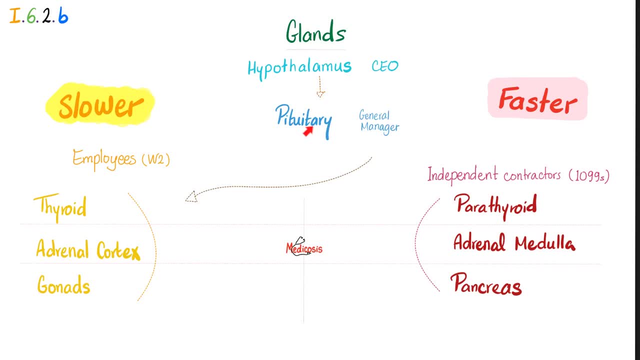 hypothalamus And then you have the epinephrine, And that's why your adrenal medulla has to be an epiphyseal portal circulation And then go to the pituitary to influence the pituitary to secrete a second hormone, And then the second hormone will be secreted into the bloodstream, It will flow. 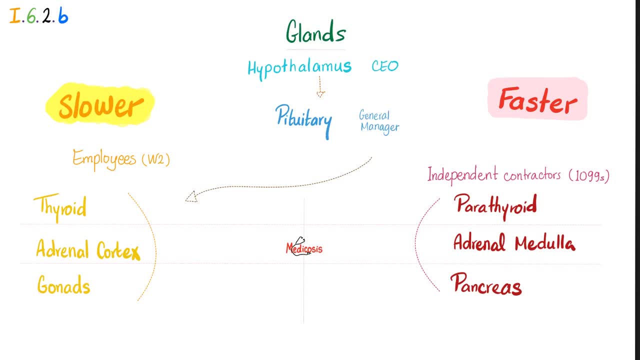 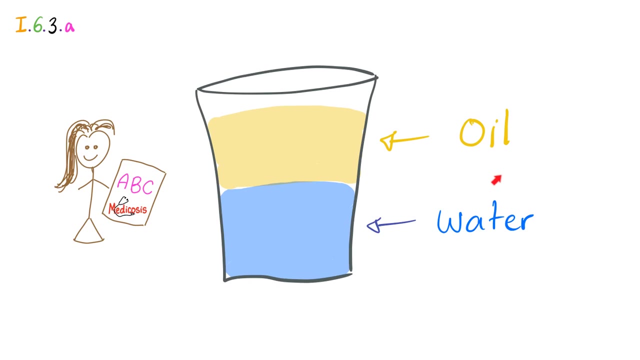 flow, flow in the bloodstream and then leave its plasma protein and then jump on the receptor, And after this I will act. the tiger would have eliminated your butt, But for intercourse you can wait. Analogy number three: the classic school experiment: water and oil. Of course water and. 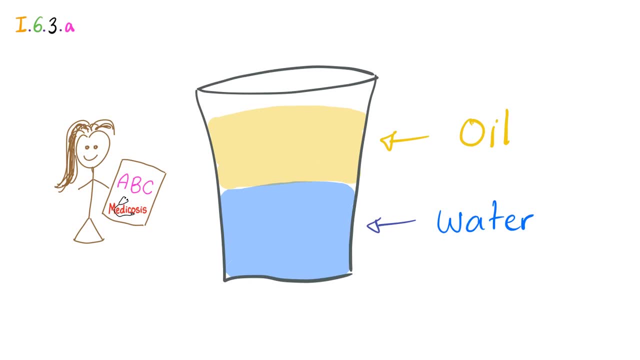 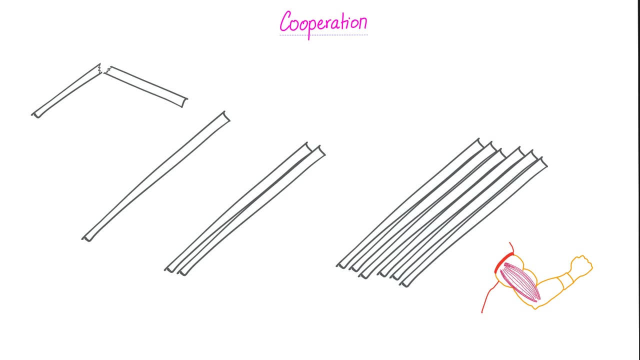 oil, do not mix. A famous Egyptian president once said. I also reminisce about the story that they used to tell you in school. Remember you get one stick, OK, try to break it. Oh easy, I can break it, But then 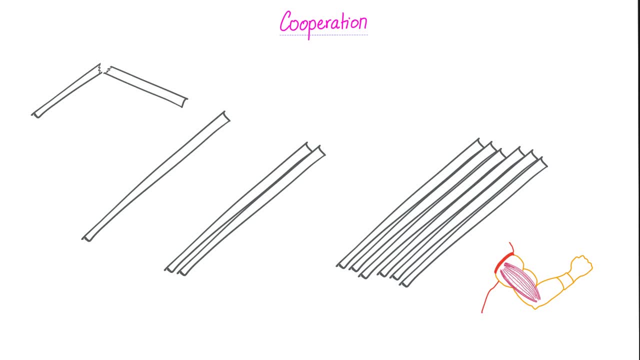 if we make a bundle of sticks, you will not be able to break it until your teacher gives this bundle of sticks to a very muscular student. The muscular student will break all of them at once And then the teacher will say: the moral of the story is: as long as this doofus is with you, 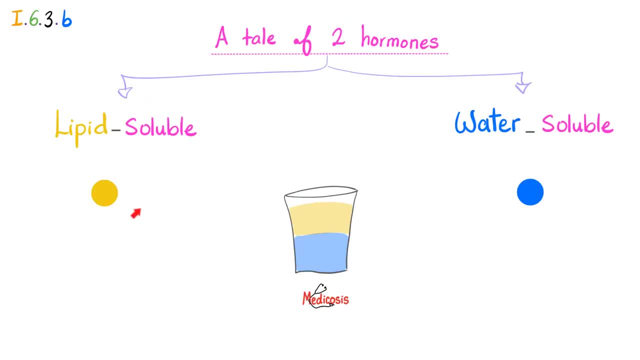 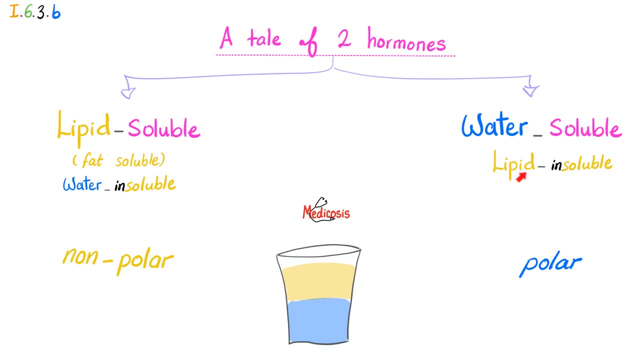 you'll be OK. So you have two things that are the same thing. You have lipid soluble and water soluble. Lipid soluble or fat soluble, of course, are water insoluble. No kidding, Water soluble are lipid insoluble. We call those nonpolar and those polar. Remember hydrochloric acid, for example? Once you 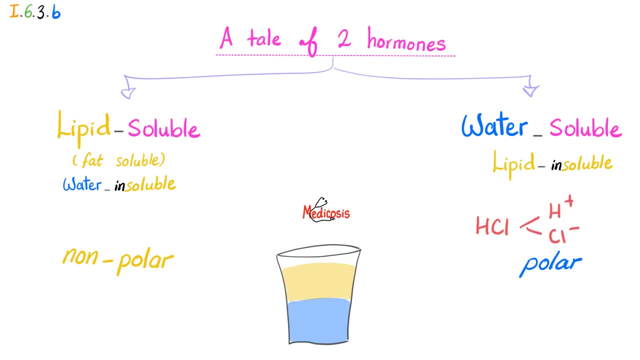 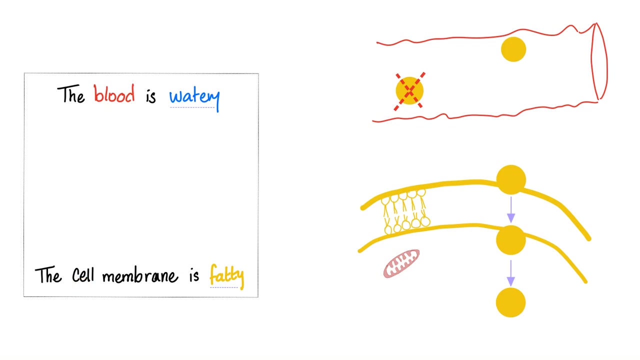 put it in water. it's going to give you hydrogen positive and chloride negative. This is polarity. You have a positive pole and a negative pole. Put some oil in water. It does not dissociate into negatives. Why do I care? Let me finish. Your blood is watery, but your cell membrane is fatty. Oh, 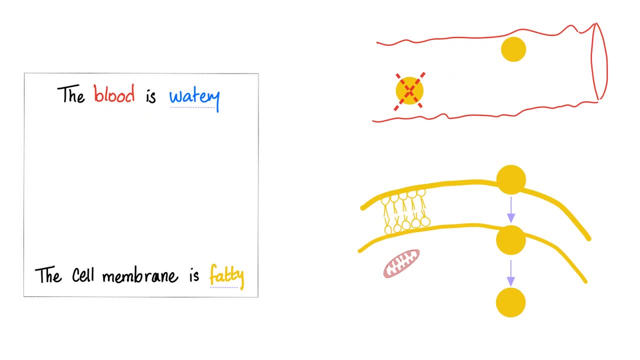 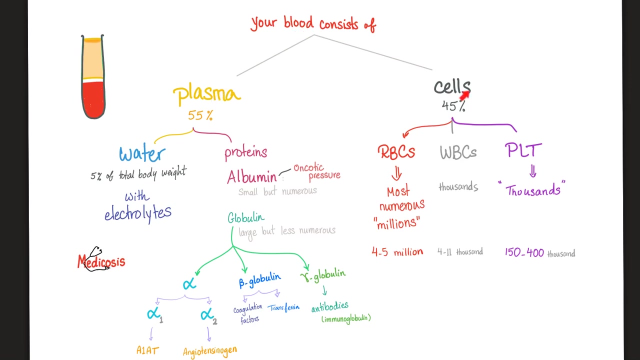 like: yeah, really, Your blood, your plasma is made of plasma. Yeah, And the plasma is basically water. Water is two thirds of your human body. The cell membrane, however, is fatty. It was made of phospholipid. It was a lipid bilayer, Let me remind you. your blood had plasma and cells. The 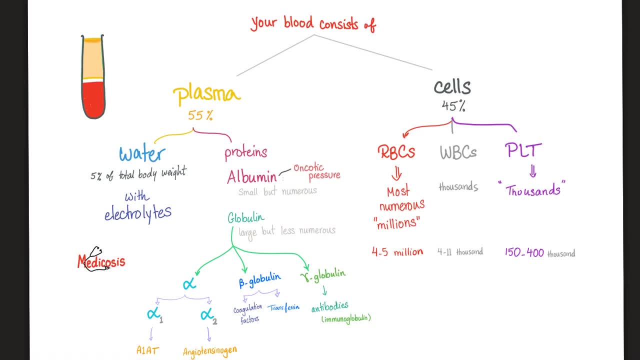 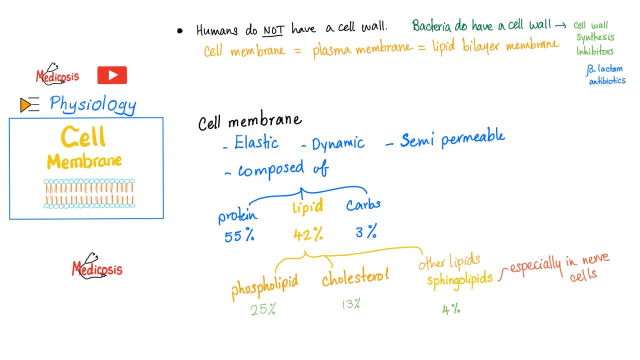 plasma had water and proteins such as albumin and globulin. Your blood is watery. However, your cell membrane is oily. It's as oily as the index finger of a junkyard mechanic. It has tons of lipids: phospholipid, cholesterol and other lipids such 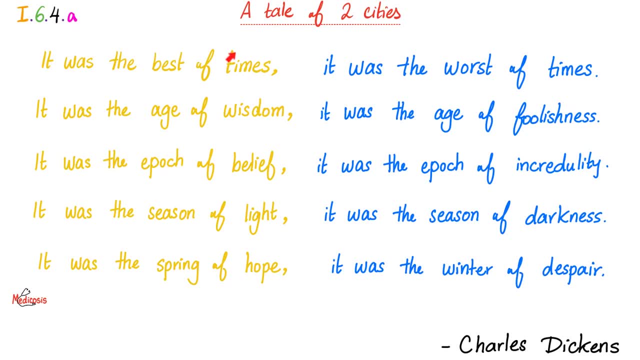 as sphingolipids. Analogy number four comes from A Tale of Two Cities by Charles Dickens. It was the best of times. It was the worst of times. It was the age of wisdom. It was the age of foolishness. 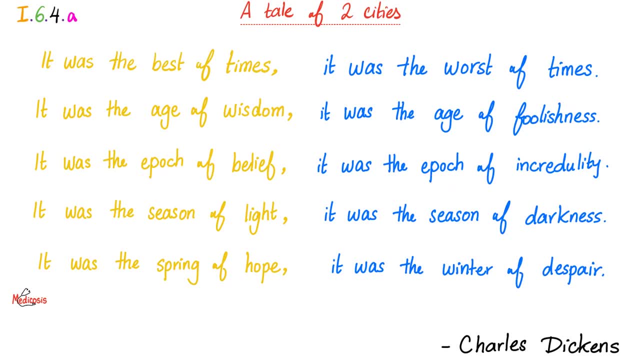 It was the epoch of belief. It was the epoch of incredulity. It was the season of light. It was the season of darkness. Oh, I wish I was born in Boston. It was the spring of hope. It was the winter. 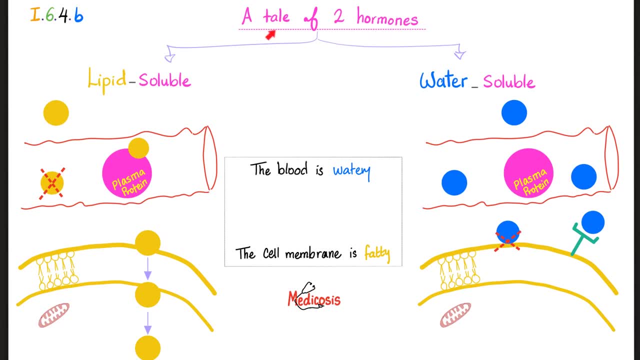 of despair. In endocrinology, you have a tale of two hormones: the lipid soluble and the water. They are different. Let me explain. Lipid soluble: Okay, I'm lipid, I'm fatty. Your blood is made of water. Therefore, I cannot float in the blood because this is lipid and the blood is water. 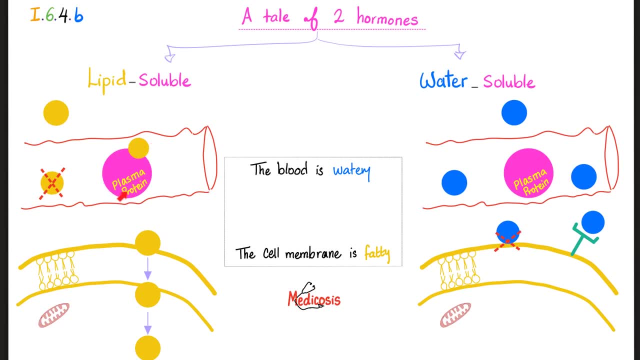 They do not mix. However, you can carry me on a plasma protein while I'm in the blood, But once I live in the water, I can't float in the blood. I can't float in the blood. I can't float in the blood. 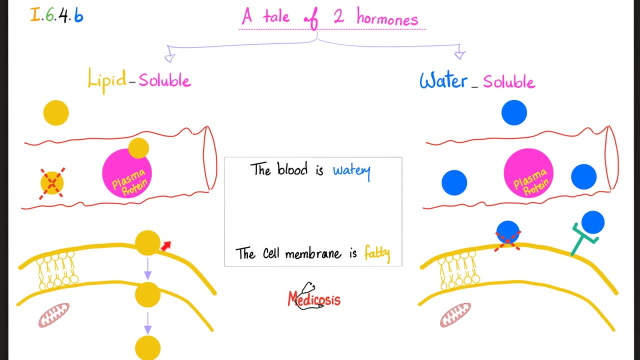 If I leave the blood and go into the cell, the cell membrane is fatty. It's oily as me. Therefore I can just squeeze through it, Simple diffusion. On the other hand, water soluble hormones. they are watery and your blood is watery. Therefore there is no need for plasma protein. They are 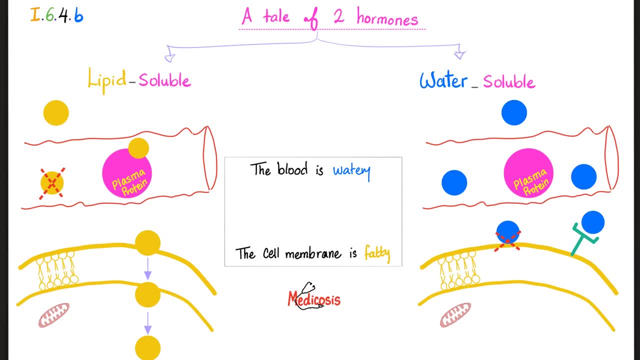 freely floating in the bloodstream, But once they reach the cell, they will not be able to diffuse. Oh, because the cell membrane is fatty, But this is water soluble. Therefore, you have to put the receptor on the outside surface, not on the inside, because it will not be able to enter The 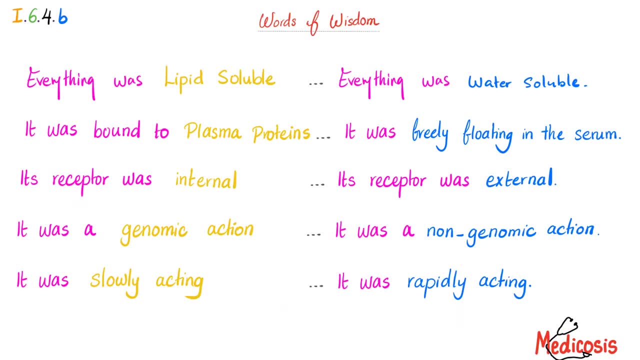 receptor has to be waiting on the outside. So let's compare between lipid soluble hormones and water soluble hormones. Everything was lipid soluble, Everything was water soluble. It was bound to plasma proteins. It was freely floating in the serum. Its receptor was internal Its. 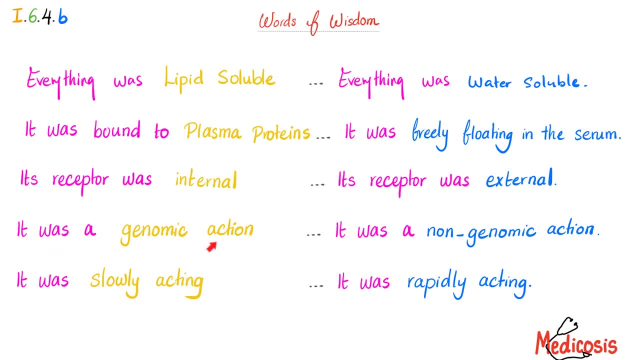 receptor was external. It was a genomic action, meaning since I was able to enter the bloodstream, enter into the cell, I will influence DNA, RNA, protein synthesis, etc. But this one, the receptor, is on the outside. This is a non-genomic action. It has nothing to do with genes. It was. 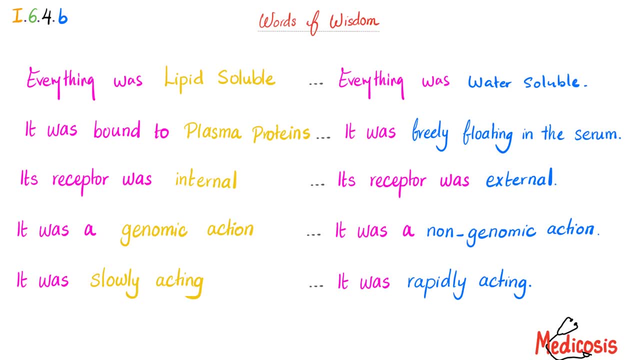 slowly acting? yeah, because I have to be carried on a plasma protein And then, once I reach the cell, I have to leave the plasma protein And then I have to diffuse through the membrane, which takes a lot of time. I'm slowly acting, But water soluble is rapidly acting, So which way of learning is? 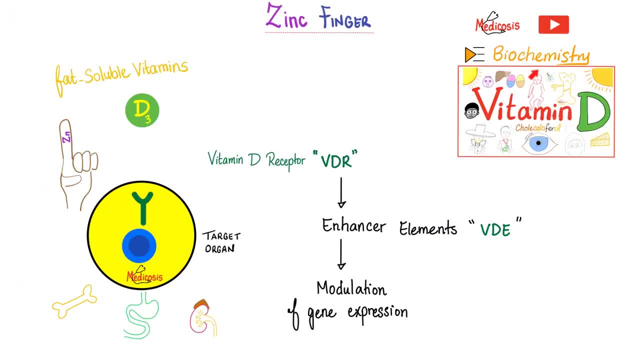 your world professor reading a PowerPoint. If you remember my biochemistry video on vitamin D, I've told you about the zinc finger. Vitamin D is a fat-soluble vitamin. Therefore, it will be able to pass and diffuse through the cell membrane via simple diffusion And therefore the receptor. 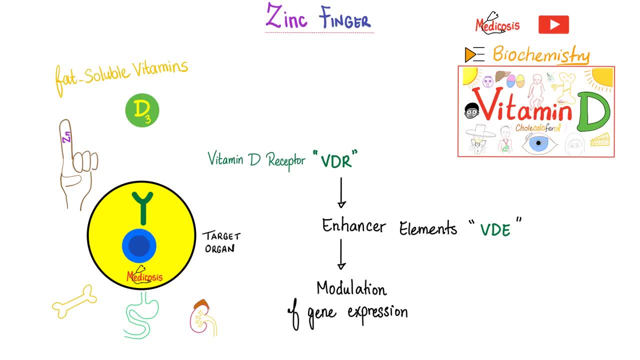 is not on the outside, It's on the inside, could be on the nucleus or in the cytoplasm, Alright. And then, once it binds to the receptor, we have the genomic action, You have some genes and we have VDR, vitamin D receptor, VDL. It's all about the overall life cycle, Because we are going to have to. 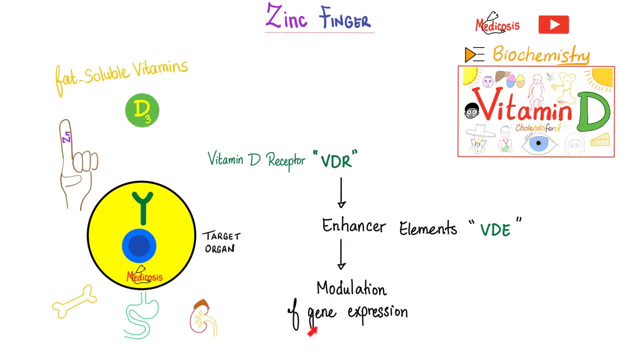 make it a little bit more complex and a little bit more complex. It's going to take just a few days to have a little bit more time to do that And, as I said, the hydrogen vitamin D is pretty much in the room receptor enhancer elements and this modulates gene expression. You have transcription and: 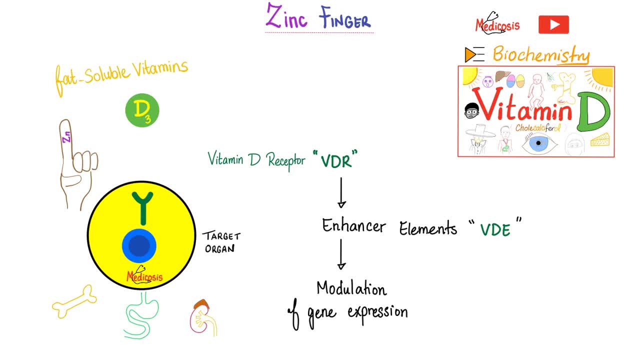 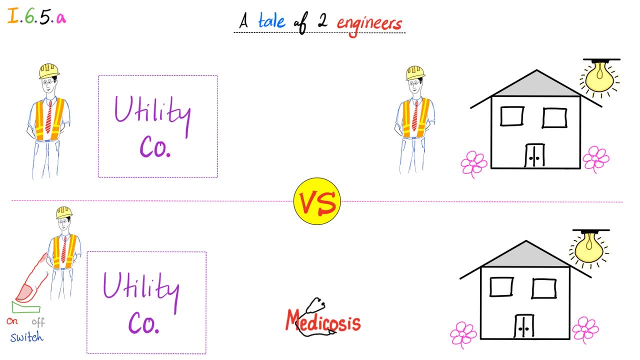 translation. Transcription is to make RNA, Translation is to make proteins. Analogy number five: Imagine that you are an engineer working for a utility company and you decided to turn the electricity off in this house, like they did in Texas. Terrible joke, I'm sorry. Which method? 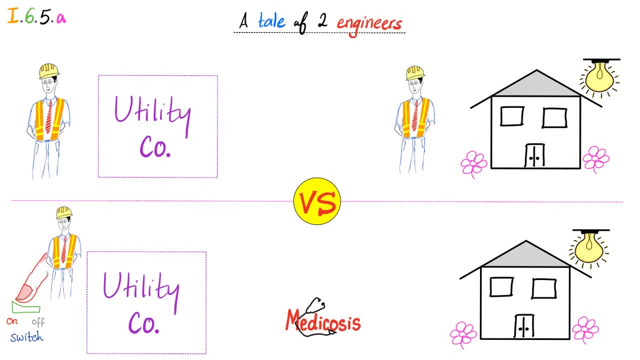 is faster: For the engineer to just flip a switch or for the engineer to leave his office at the utility company and then drives his car on the highway and then goes to your house, knocks on your door, tips his hat, kisses your wife- I mean kisses your puppy- and goes to town, climbs over. 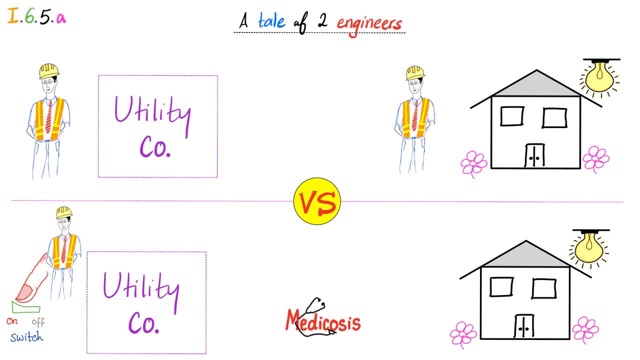 the ladder that you got from Home Depot using your credit card because you could not afford it, you cheap bastard. and then unscrew the light bulb. Which one is faster? Of course flipping a switch is faster, Childish as this might seem. it's very important for endocrinology because 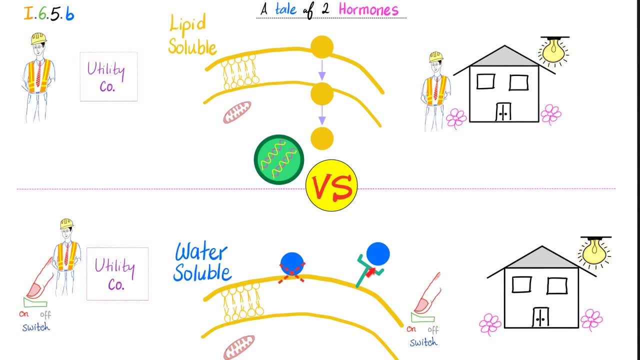 water-soluble, they just flip a switch. once they bind to the receptor that's on the outside surface, They just flip a switch. It is a rapidly acting hormone. but a lipid-soluble hormone has to wait until it unloads from the plasma protein and then it goes to the cell membrane, touches the membrane. 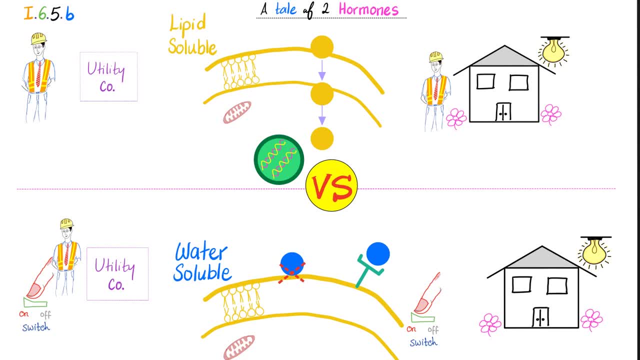 and then diffuses through the membrane, which takes time- This is fat inside of fat- and then diffuse through the cytoplasm And then try to find the receptor. The receptor could be in the cytoplasm or could be on the. 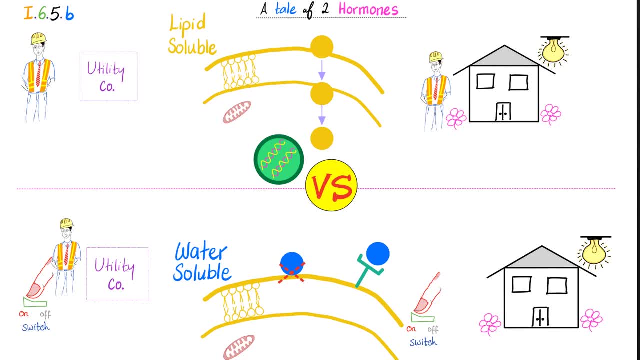 nucleus. Of course, this is slow acting And that's why, when you're running from a tiger running for your life, your adrenal medulla had to not obey the pituitary. It had to secrete a water-soluble hormone known as epinephrine or norepinephrine, so that we can just flip a switch. 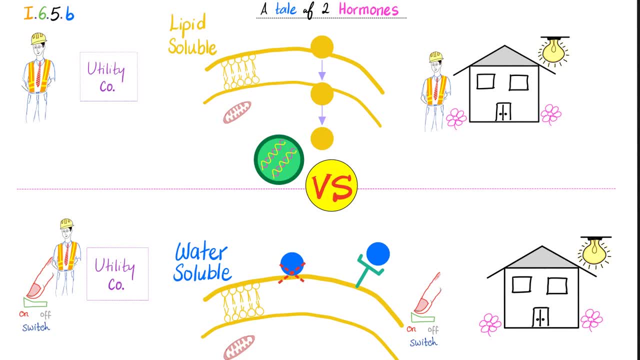 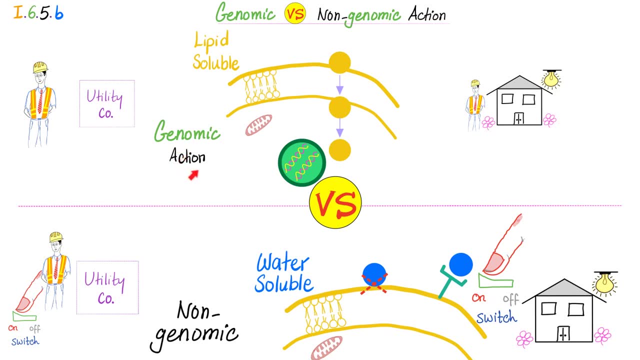 But if you want to participate in coitus, take your time, take it slow. Hashtag serendipity. And that's why we say that lipid-soluble hormones have a genomic action: because they influence gene, because the receptor is on the nucleus or in the cytoplasm. We will influence and stimulate. 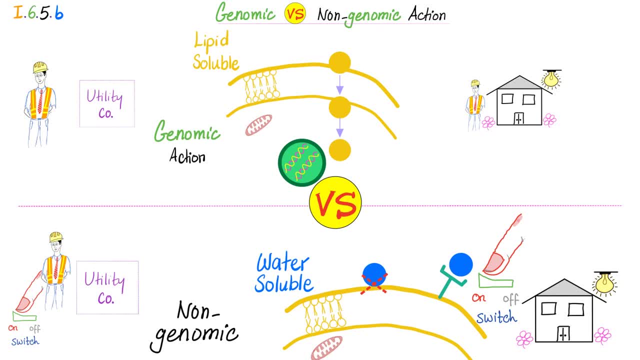 gene expression and then DNA transcription and then into RNA and then translation or protein synthesis from the RNA. However water-soluble, they just flip a switch. It's a non-genomic action. They do not synthesize new proteins. 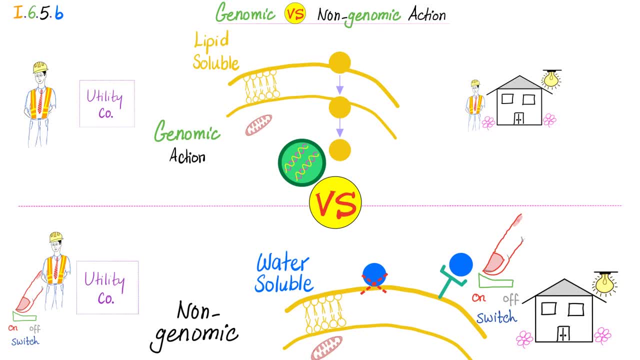 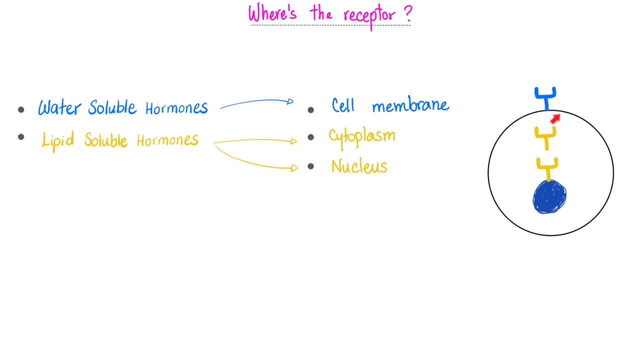 They just replace previously synthesized proteins. That's why they are rapidly acting. So where would you put the receptor? Would you put it on the cell surface? Would you put it in the cytoplasm or on the nucleus? Well, it depends. If you're water-soluble, you will not be able to. 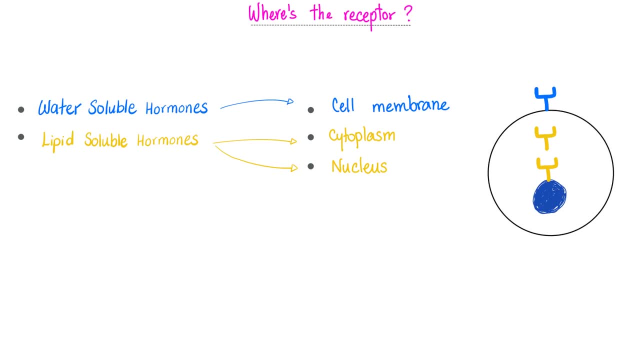 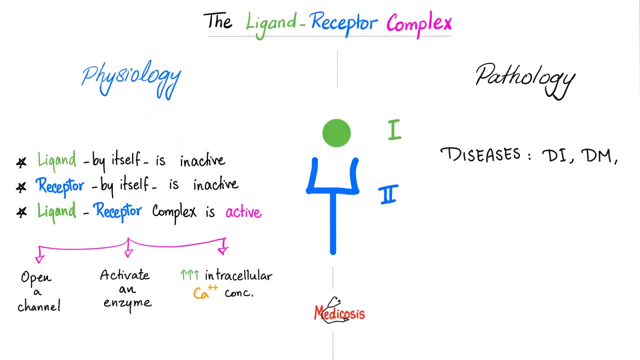 enter. Therefore it has to be on the outside. If you are lipid-soluble, however welcome, Come on in. I put it in the cytoplasm or the nucleus. Here is another story, The story of the key and the lock. 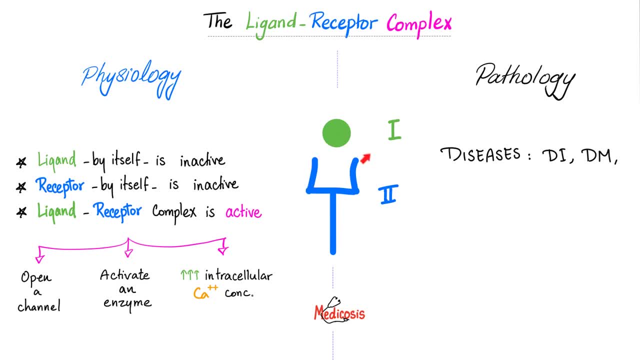 The truck and the dock, The ligand and its receptor. A specific ligand has a specific receptor. The ligand on its own is inactive. The receptor by itself is also inactive. Only the ligand-receptor complex is active, Only when the key goes deep inside the lock. only then is it active, Only when the truck 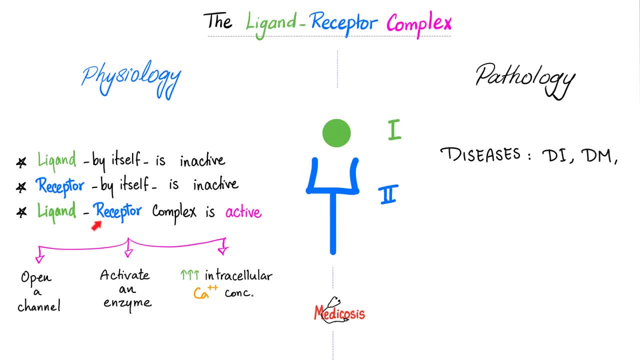 hits the dock, can you start shipping? So the ligand-receptor complex is active. Active to do what? open a channel and hire Piers Morgan, activate an enzyme or increase intracellular calcium concentration. Okay, this is normal. What is pathology? Well, pathology is a disease such 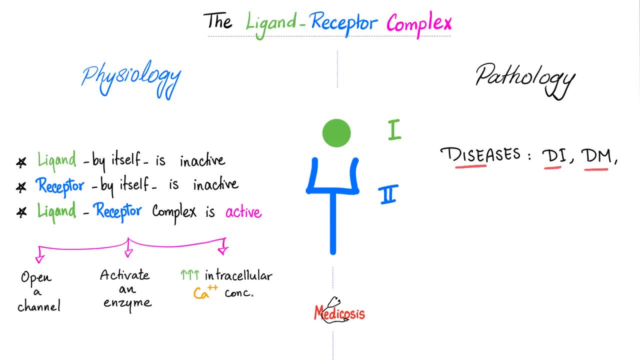 as diabetes insipidus, diabetes mellitus. And what's the problem here? Well, the problem could be here, and we call this type 1 diabetes mellitus or central diabetes insipidus. or the pathology could be here, in the receptor, and we call this type 2 diabetes or nephrogenic diabetes insipidus. 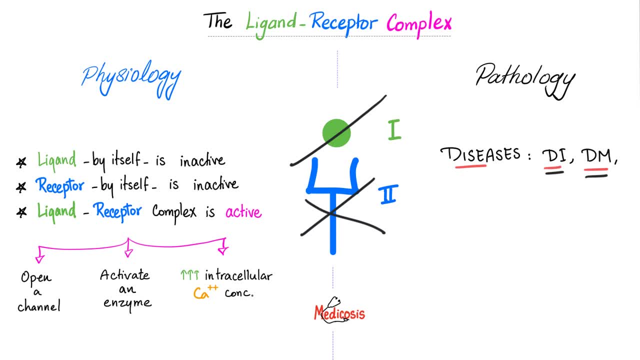 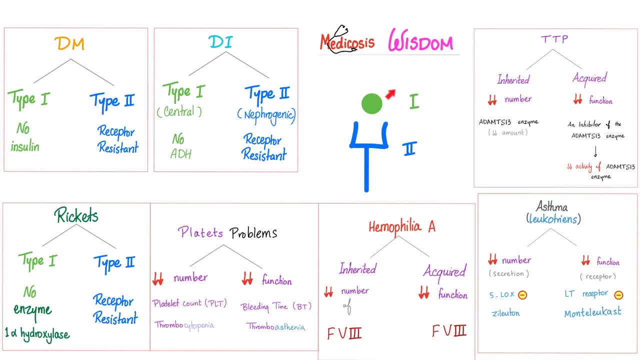 Pathology can hit your ligand or it can hit your receptor. Either way, you will be inactive, and this is the definition of disease. There is no more ease. So in medicine, whenever you hear about type 1 or type 2, usually here is what we mean. Type 1, the problem is in the hormone Type. 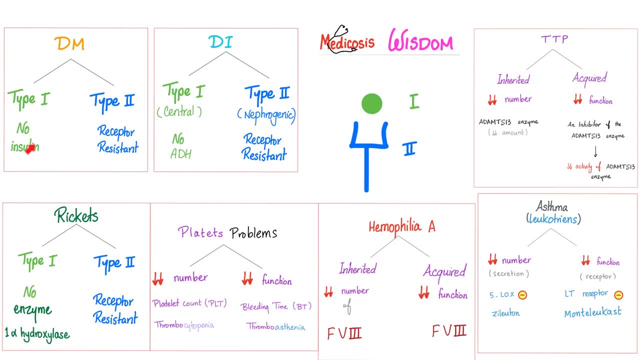 2, the pathology is in the receptor. Example: diabetes, type 1, no insulin. The hormone is gone. How about type 2?? Well, there is some insulin, but the receptor is not listening. The problem is in the receptor called the resistant. 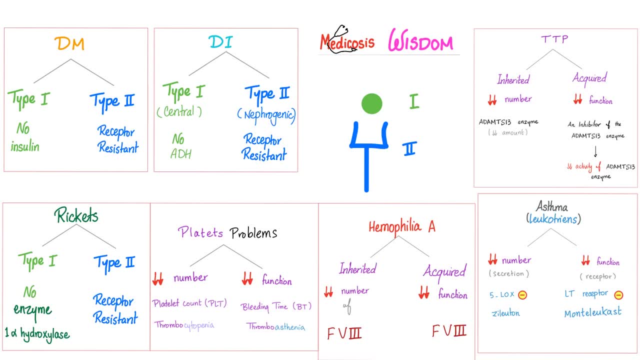 or insensitivity, Diabetes, insipidus? we have type 1, or central, no ADH. How about type 2?? Well, there is ADH, it's just the kidney's receptor is not responding. How about trichids? Type 1,? 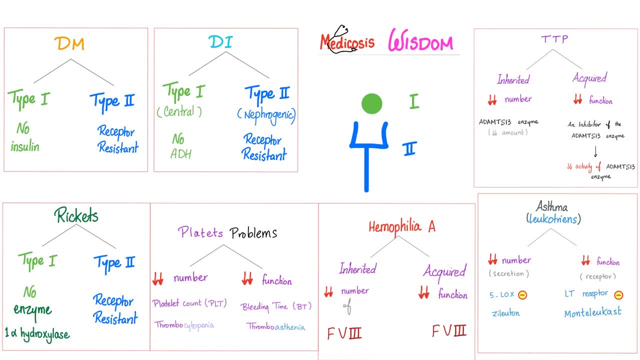 there is no enzyme, there is no 1-alpha-hydroxylase Type 2, receptor resistant. And then we have a similar situation with platelet Problem: decrease number, decrease function, Hemophilia A, decrease number of the factor. 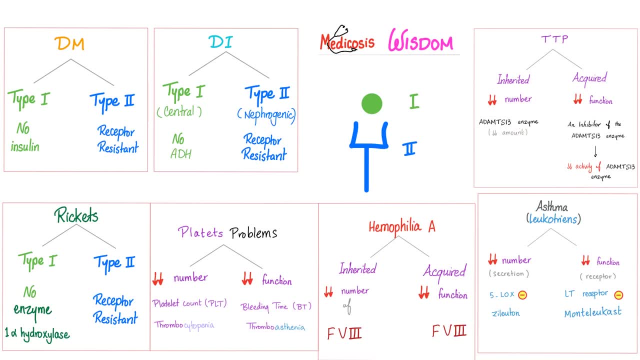 decrease function of the factor TTP. decrease number, decrease function. How about leukotrienes? How do you treat asthma? You treat asthma by decreasing the number of leukotrienes or decreasing the function. You can either inhibit the secretion of leukotrienes or inhibit the 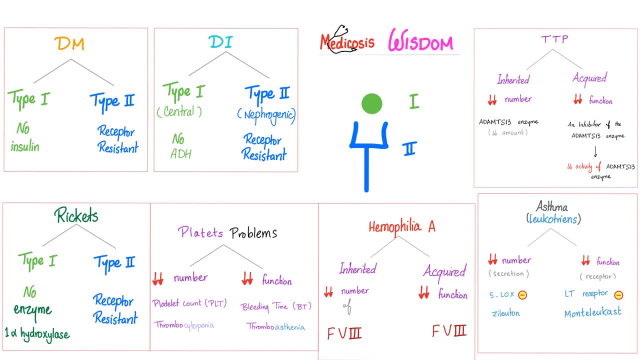 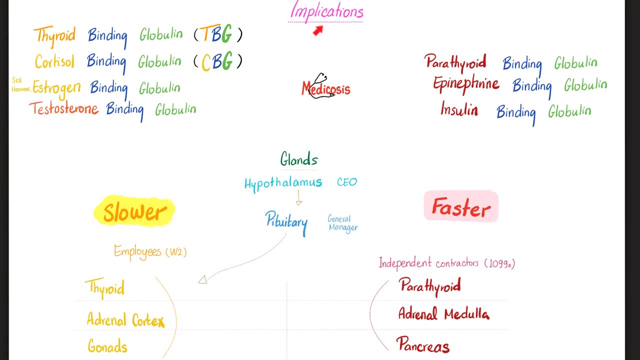 receptors of leukotrienes. The first is called xylutin. the second medication is called the montelocast And we have talked about this before in my pulmonology Playlist Implications. All right, remember the CEO and the general manager, and we have three. 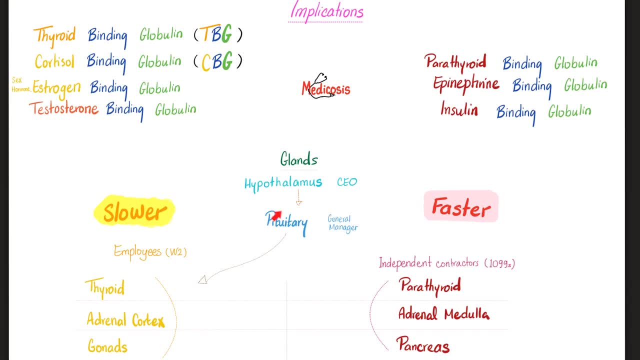 employees that listen to the pituitary and the hypothalamus. Okay, These hormones that listen, of course, are slower. Yeah, because we have to wait, And since they are slower, they are fat-soluble. Yes, because lipid-soluble hormones are slow. Lipid-soluble hormones have to wait. until they unload from the plasma protein, until they diffuse through the cell membrane. But water-soluble do not. Fat-soluble hormones are carried on plasma protein Why? Because they are fat-soluble and your blood is made of water. 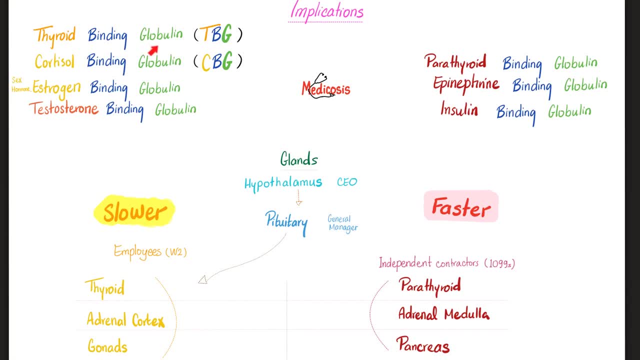 You cannot float in the blood. if you are made of fat, I have to carry you on a plasma protein. Which type? Could be albumin, could be globin, And that's why we talk about thyroid-binding globin in the lab: cortisol-binding globin, estrogen-binding globin or testosterone-binding. 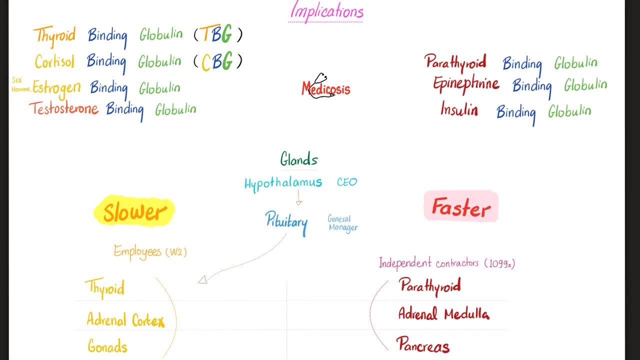 globin, or you can call them collectively sex hormone-binding globin. If you understood this lecture so far, this is going to be a piece of cake. The reason why you don't understand medicine is shaking. Conversely, have you ever heard of a parathyroid-binding globin? epinephrine-binding? 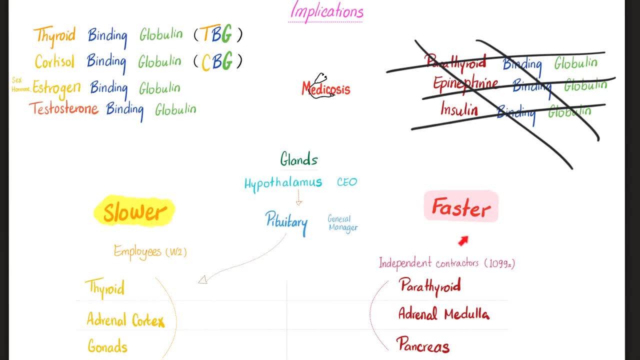 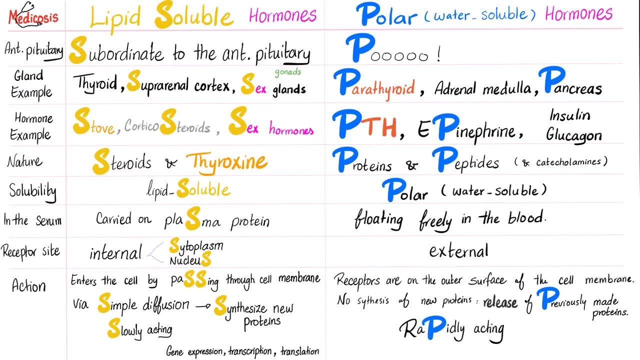 globin or insulin. They do not exist. Why not? Because they are water-soluble, They are faster. These are the independent contractors, And here is a beautiful table that can help you cruise through endocrinology like a sharp knife in warm butter: Lipid-soluble versus water-soluble. 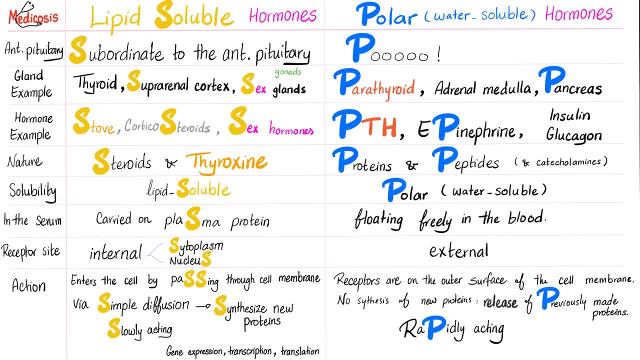 hormones? Lipid-soluble- Okay, what are they? They are subordinate to the end-tube pituitary. They listen and obey, But polar poo-hoo pituitary, who cares? Lipid-soluble: Can you give me an example of glands that secrete these lipid-soluble hormones? 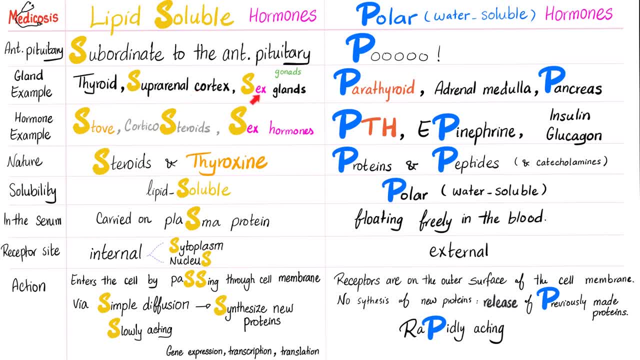 Sure, Thyroid, suprarenal cortex and six glands or gonads. Okay, what do they secrete? Thyroid gland will secrete the thyroid hormone, or what I call the stove of the body, because everything will be on fire. It increases your metabolism, it increases your heart rate, it increases your 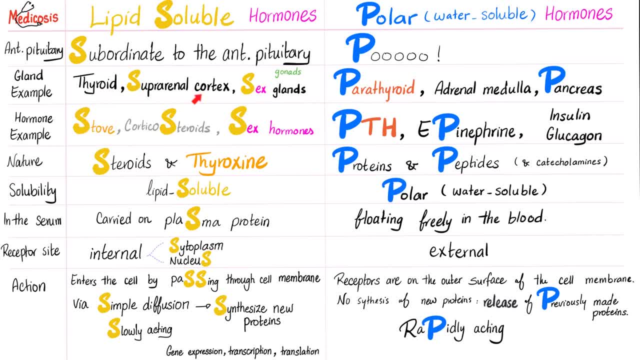 gastric motility, bowel motility, everything. What does the suprarenal cortex secrete? The corticosteroids, especially cortisol. How about the six glands or the gonads? They secrete sex hormones, so that you can participate. 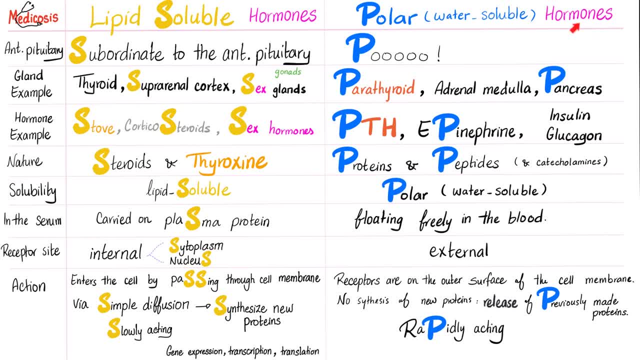 in coitus. These are good times right there. On the other hand, the glands that secrete polar hormones include parathyroid gland, adrenal medulla, not cortex medulla and the pancreas. What does the parathyroid gland secrete? Parathyroid hormone? How about adrenal medulla? 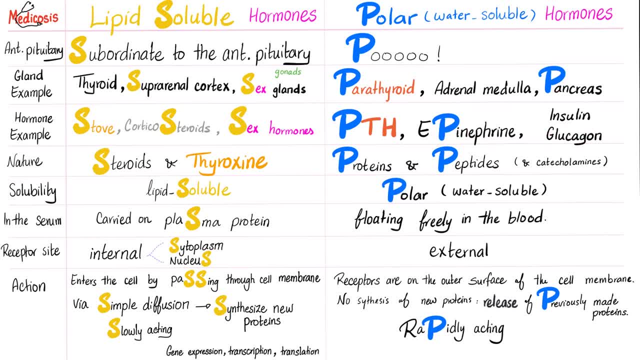 epinephrine or epinephrine, etc. Pancreas insulin, glucagon and somatostatin. Next, what's the nature of these lipid-soluble hormones? Well, they are lipid-soluble. 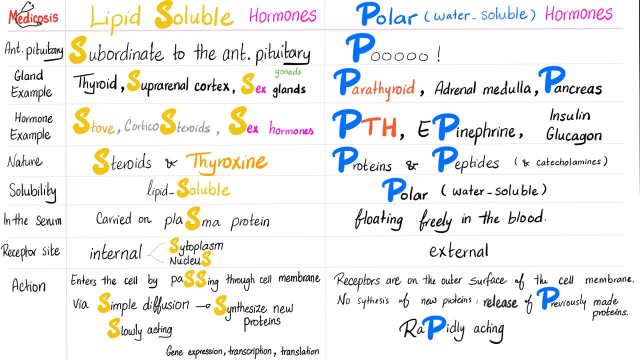 they are steroids and thyroxin. These are collectively lumped together. How about the polar hormones? These are proteins, polypeptides, peptides and catecholamines. We lump them all together. Okay, solubility- I am lipid-soluble, of course. How about these ones? They are: 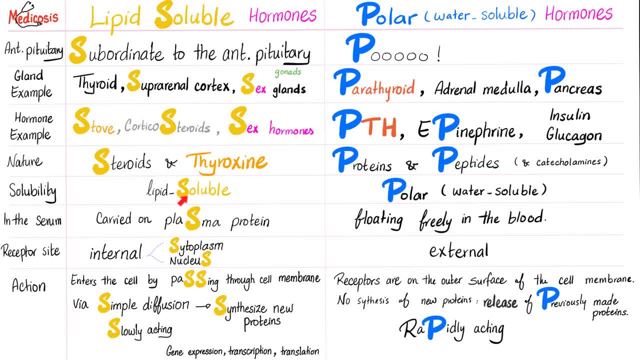 water-soluble. Therefore I cannot float in the serum because the serum is watery and I am oily. You have to carry me on plasma protein. but now I'm polar, Ah I poo-hoo. I can float freely in the blood. You can say P for passive. 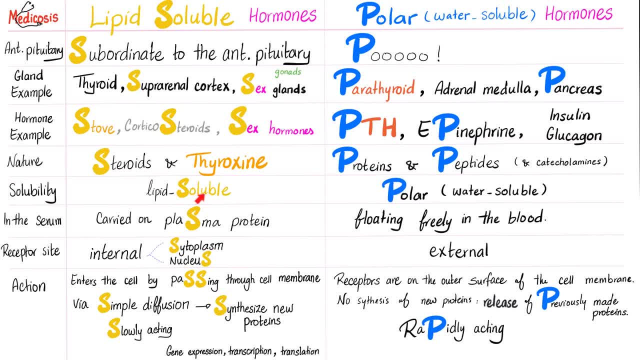 Since you are lipid-soluble, where is your receptor? Well, I will enter into the cell by diffusing through the cell membrane. Therefore, you can put my receptor in the cytoplasm or the nucleus. Okay, how about you polar? Ah, you have to put it on the outside because I cannot enter. 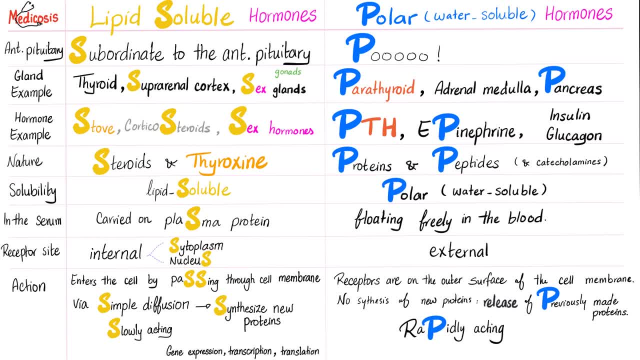 because I am water-soluble, Action All right. I'm lipid-soluble, I'm carried on plasma protein. I will enter the cell by passing through the cell membrane, via simple diffusion, and I will synthesize new proteins by expression, transcription, translation. This is a slow process, Conversely water-soluble hormones. 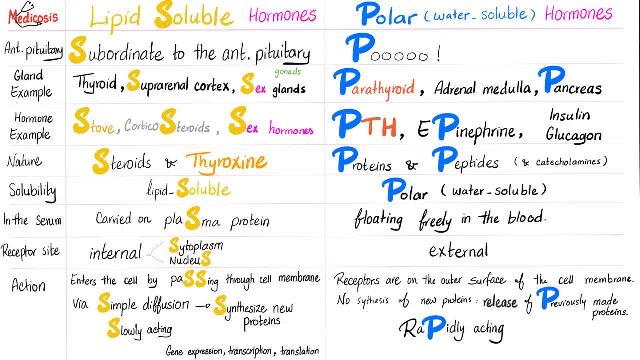 the receptor has to be on the outer surface of the cell membrane. Okay, there is no synthesis needed of new protein. You just release previously made proteins, and this is a rapidly acting hormone. Let's look at it in another way. Lipid-soluble hormones are steroids and thyroxin. Okay, 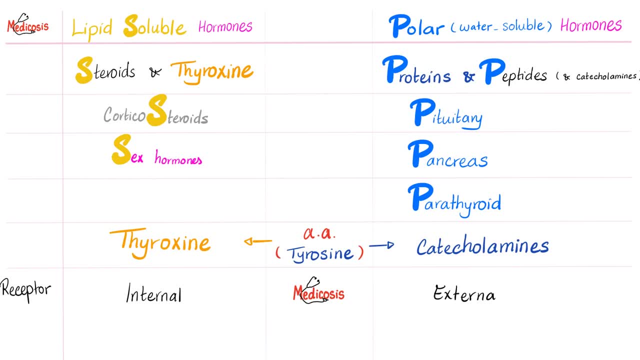 they are corticosteroids and sex hormones, All right. where did thyroxin come from? It came from amino acid called tyrosine. Okay, thank you. How about polar hormones? You have proteins and peptides and catecholamines. 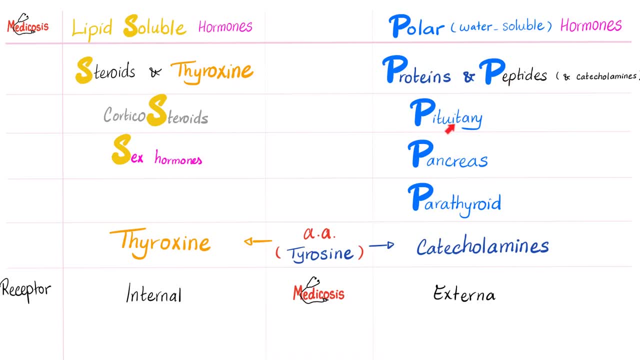 Awesome. They come from the pituitary, so most of the hormones that come from the pituitary are water-soluble. How about the pancreas Water-soluble, Parathyroid Water-soluble? Where did the catecholamine come from? Oh, the catecholamines came from the same amino acid, tyrosine. 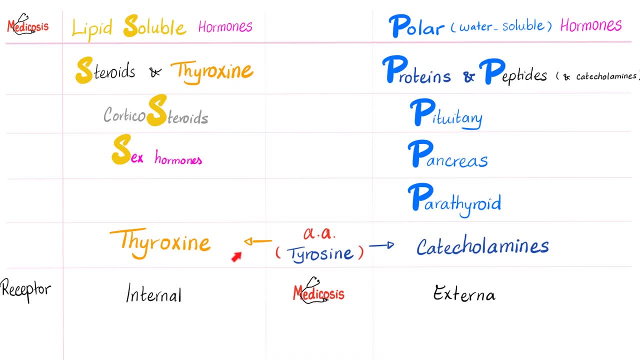 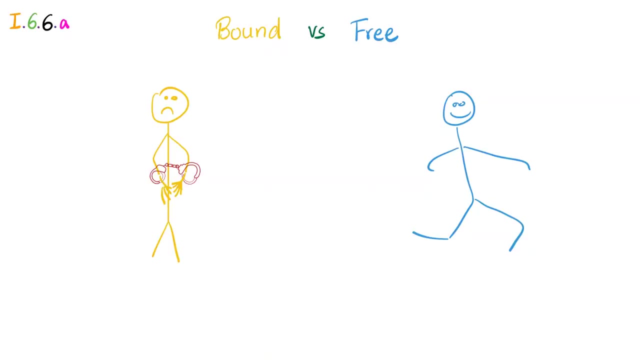 So wait, wait, wait. a second One amino acid can give rise to thyroxin, which is with this group, and catecholamines, with the water-soluble group. Absolutely, and this is important. These are called tyrosine derivatives. Story number six: Are you bound or are you free? Which one is more active? 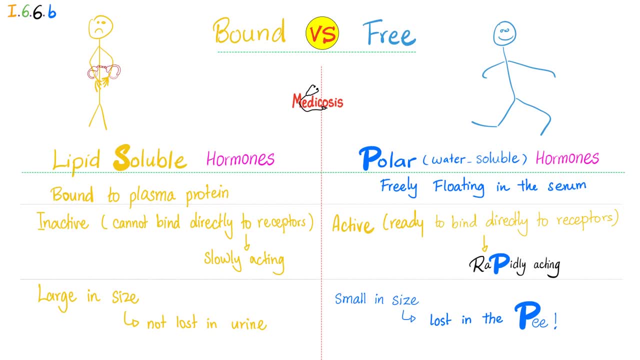 The free Lipid-soluble. I cannot float freely in the plasma because the plasma is watery and I am oily. You have to bound me to plasma protein. Since I am bound, I'm inactive. Therefore I cannot readily or directly bind to receptors because I have to unload. 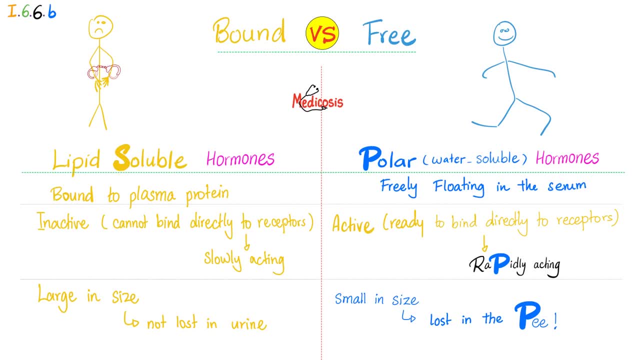 first I have to unlock from the plasma protein and then I can go to my receptors. So therefore I'm slowly acting. Since I'm bound to plasma proteins, this will make me big. Oh yeah, we are big, We are huge. We are not filtered by the glomerulus and therefore we are not lost in the urine most of the time. 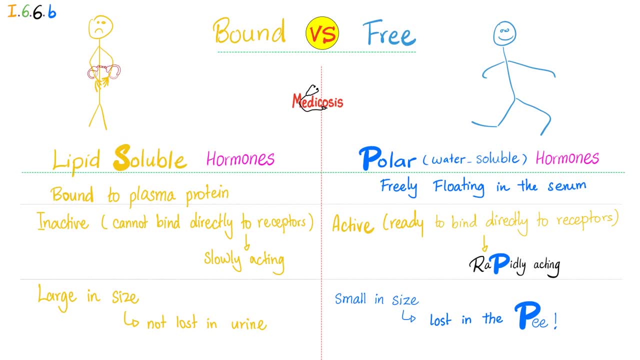 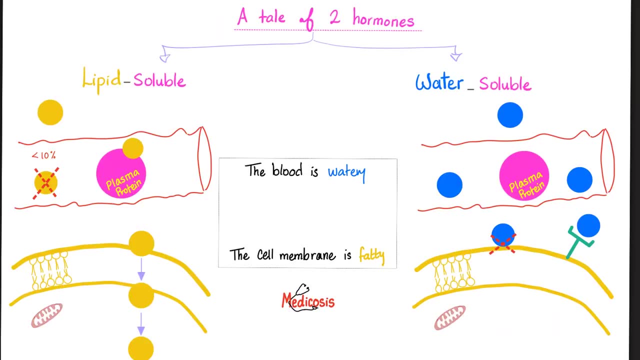 Polar hormones, on the other hand, freely floating in the serum. We are active, We are rapidly acting, We are small in size and we could be lost in the pee. Okay, medicoses, let me ask about cortisol. All right, sure, In Cushing disease, I can measure cortisol in the urine and you said that all of the cortisol is bound. 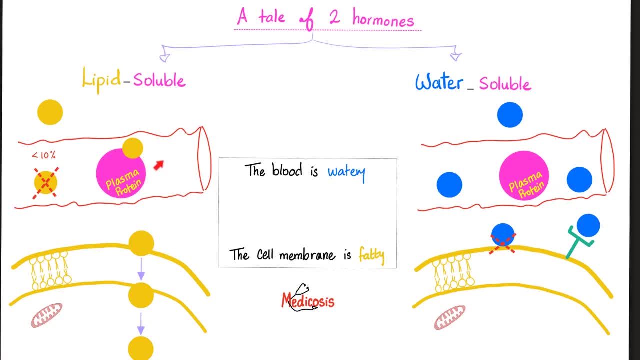 to the No, no, I did not say all of the cortisol. Most of the cortisol is bound to the plasma protein and will not be filtered. About 10% or less is freely floating in the blood. However, in Cushing disease, this 10% is greater than normal. 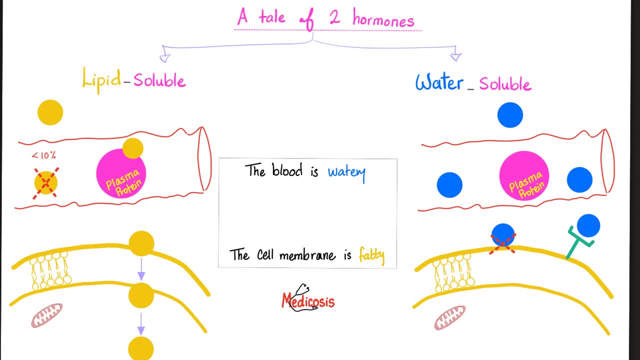 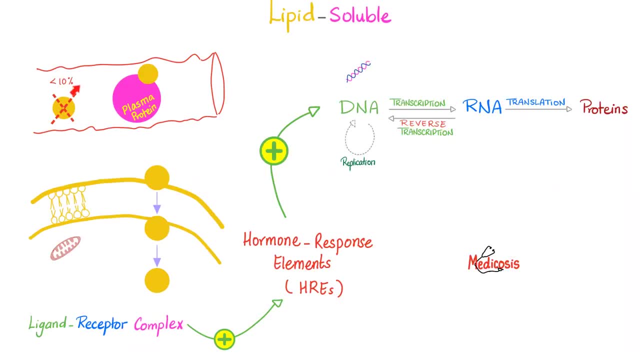 It is greater in absolute amounts and in relative amounts. So you will eventually see lots of cortisol in the urine. Let's talk about lipid-soluble- Okay, about 10% freely floating, and then the majority are on the plasma protein. 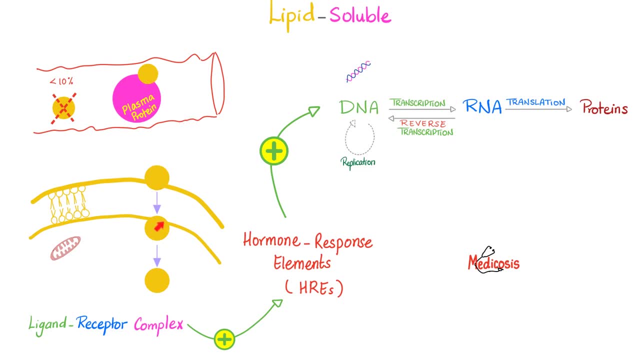 But once I reach the membrane I will unload and then diffuse. This is simple diffusion. I go inside. my receptor is in the cytoplasm or on the nucleus Ligand receptor complex or hormone receptor complex. now I'm active. 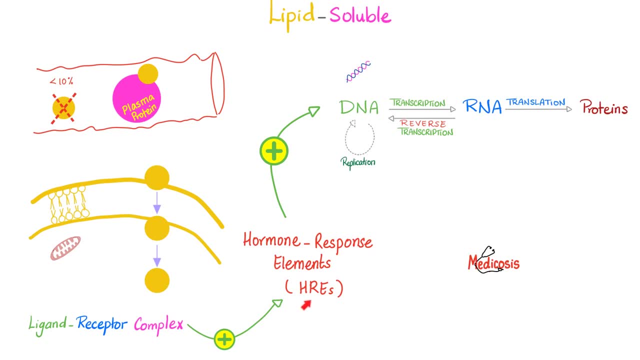 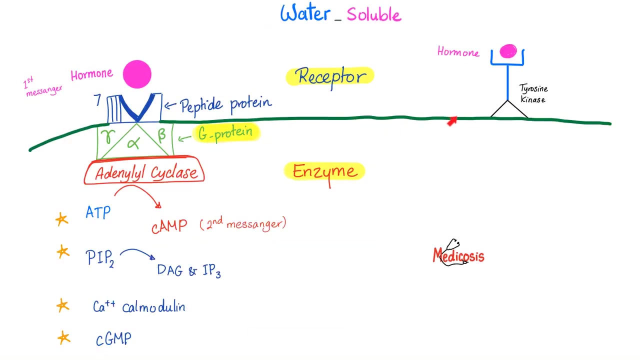 I will stimulate hormone response elements, or HREs, which will stimulate DNA. You have gene transcription, translation, all of this beautiful stuff to synthesize new proteins from scratch. How about the water soluble? I will not be able to pass through the membrane by simple diffusion. 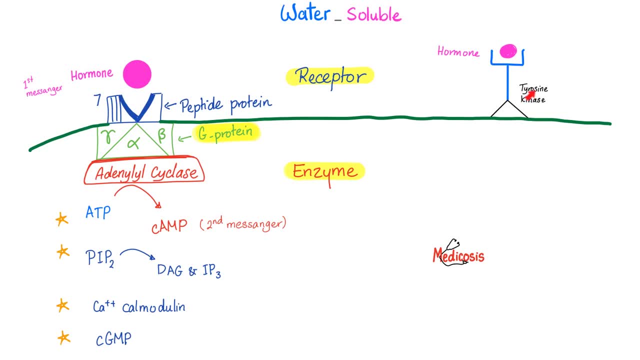 It's not gonna happen. You have to put the receptor on the outside. Okay, and this will be the story of the G protein. G protein is the switch, If you remember the engineer. G protein connects the receptor on the outside with the enzymes on the inside. 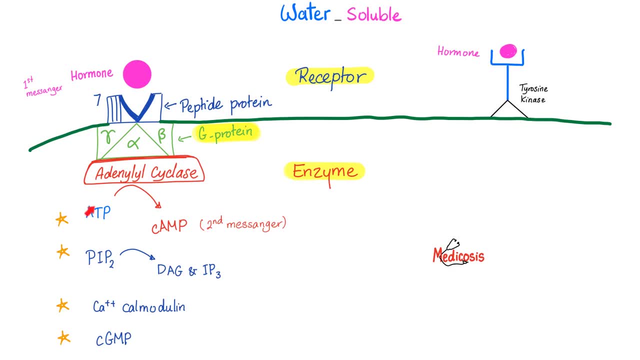 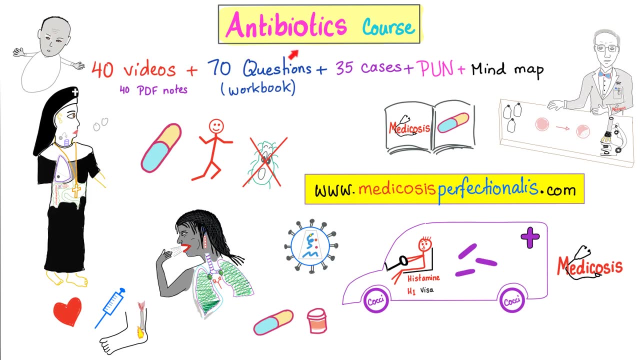 And this will be the story of the next video. We'll talk about all of the first messengers and second messengers. It's gonna be epic. If you like this video, you will adore the mother of all courses: my antibiotics course. 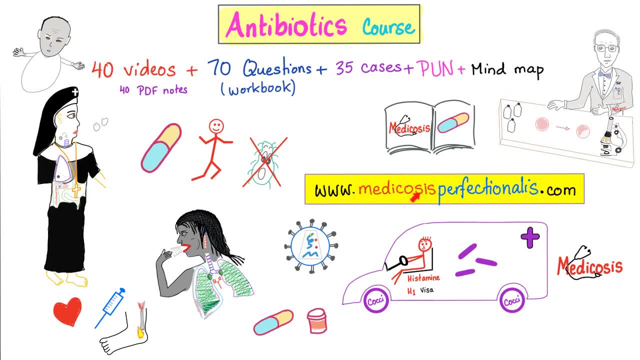 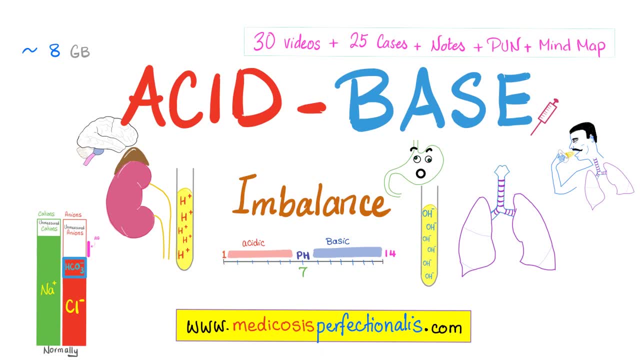 It has 40 videos and questions and cases and notes. You can download it today at medicosisperfectionalistcom. You download it once and keep it for you forever. Also, you can devour my new acid-base imbalance course. Talk about normal kidney physiology. 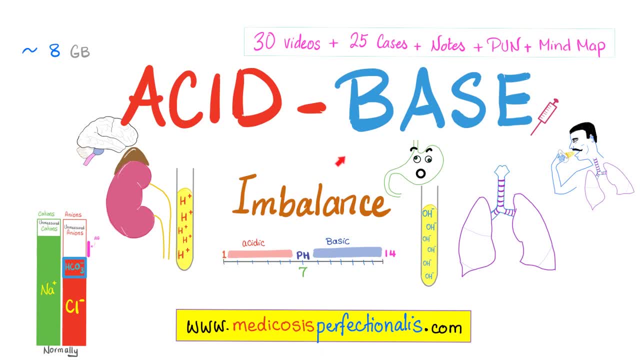 diuretic pharmacology and all of the clinical medicines and the anion gap and the osmolar gap and the serum anion gap, urine anion gap, base deficit, base excess, all of this crazy stuff and even the Henderson-Hasselbalch equation.